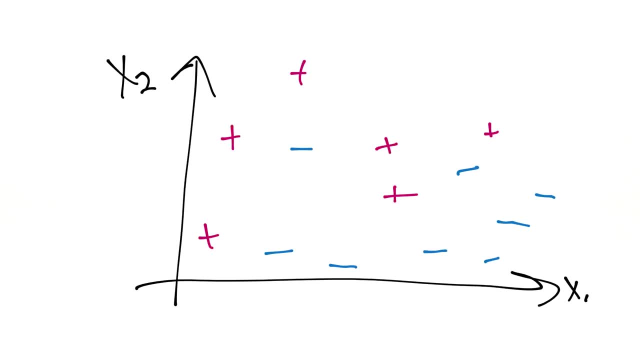 bit easier by processor, and that was only second order order, right? so in that case we had n equals two for the number of dimensions, and then p was also equal to two. but imagine it had we make made p 100 and n 1000 right? would that have made our polynomial kernel take much more processing? like 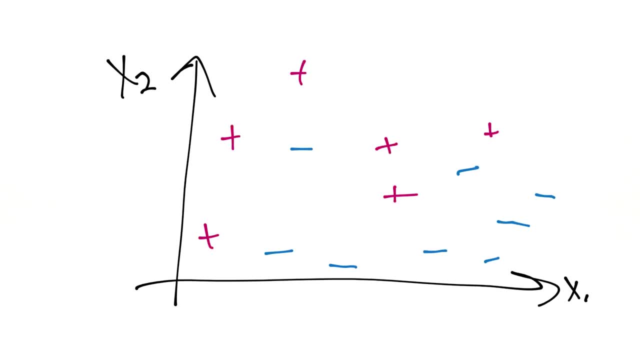 exponentially more processing? no, would it have caused an exponential increase in? uh, just actually, you know, translating to the z space and running that dot product? yes, that would have been crazy. so that's one thing we've. we kind of ended on the radial basis function kernel and explained how that can translate into. 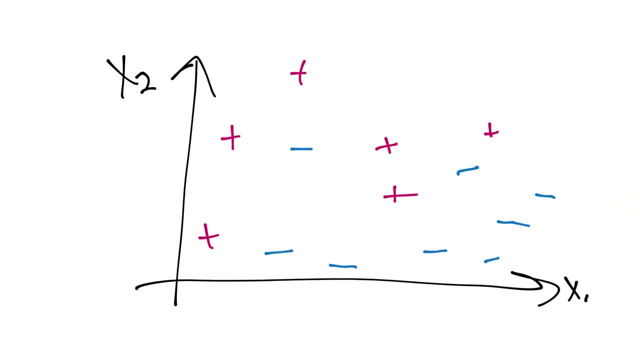 seemingly infinite dimensions, and now we're going to be talking about is where that can you know, problems that can come up when you might do something like that, and one how to know. maybe is your data actually just never going to be linearly separable, or should you maybe try? 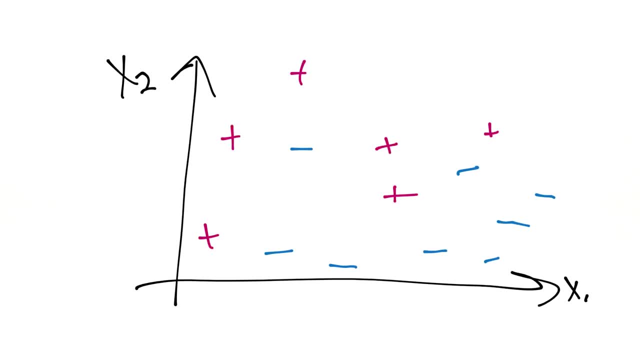 another kernel maybe, or something along those lines. so we're going to talk about that in a little bit. so that's what kind of what we're going to be talking about here. and specifically, we're going to introduce the soft margin support vector machine. so imagine you've got this data set i've drawn up. 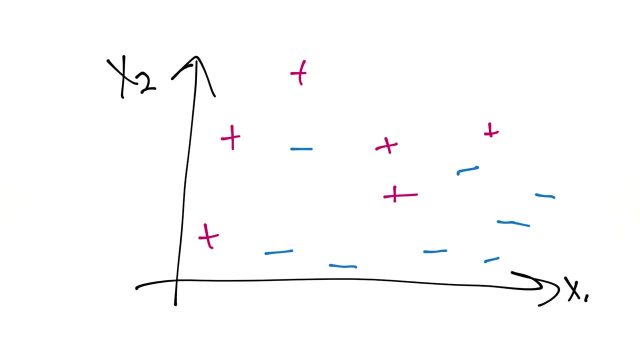 here and looking at it, you know, is this linearly separable? uh, not. no, okay right, there is no straight line that we can draw that will do this. but imagine that we run the rbf and we come up with a decision boundary. that probably looks, you know something? 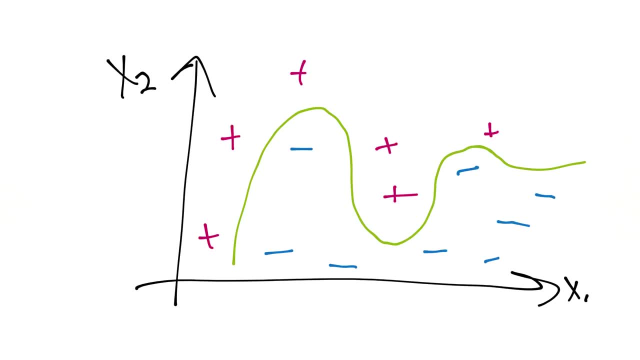 like i don't know something, something like that. right, and in this case we're going to have our- i'll do in a, in a lighter green, the, the actual support vector, hyperplane. so you know, coming through here probably comes down here, comes up here, goes out here, and then here you come down. 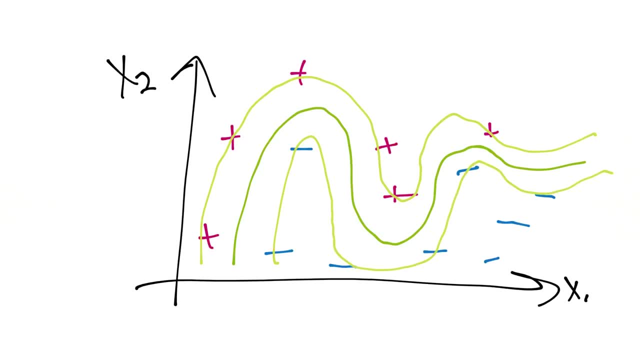 here, maybe cross into that one, this one, okay, and you go out, okay. so so that would be in theory, via the radial basis function. and now let's go ahead and just circle all of our support vectors here: bam, bam, bam, bam, bam, bam, bam: this one, this one and this one, and out of this entire data, 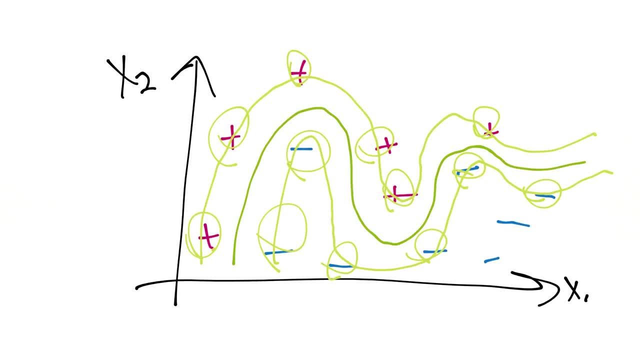 set. only two feature sets are actually not support vectors. okay, that is a major red flag. why is that red flag? well, it kind of signals that we probably have some over fitment going on here. okay, so if we can find a function that, like you know, fits the data set and we can get it to work, okay, so we can. 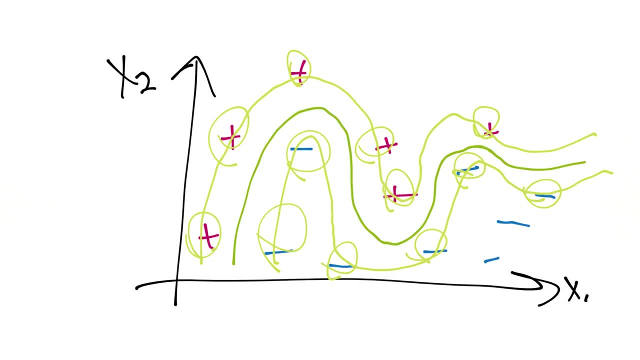 find a function that, like you know, fits the data set and we can get it to work, okay. so, if we can, all of this data, we're probably in in some trouble here. so, uh, so. so instead of maybe doing what we've just done, i will put us back to just have that, that single decision boundary. uh, what if we drew? 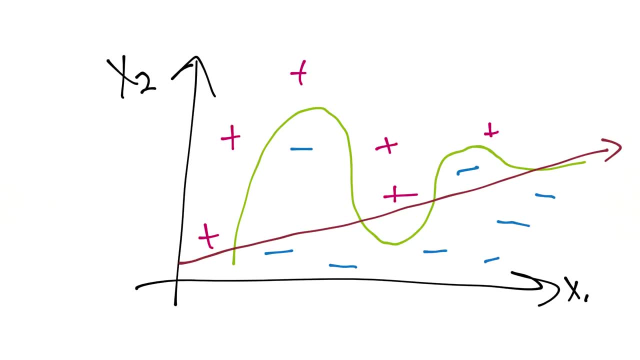 another one that right, a almost, you know, basically a straight line that separates the data, and if we're to look at this, we can see, okay, we've got, uh, a few violations. right, you've got maybe this violation here, this is a violation, and basically, yeah, that's just those. sorry, i punched my 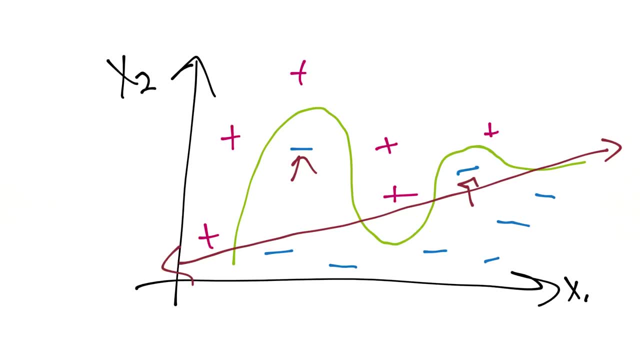 microphone punch you guys. so so you've got these two violations here, otherwise everything else fits this line. and again, what if we actually drew the, the support vector hyperplane again? we'll just kind of make it a little lighter. uh, we go here and then probably here right. and again, if we 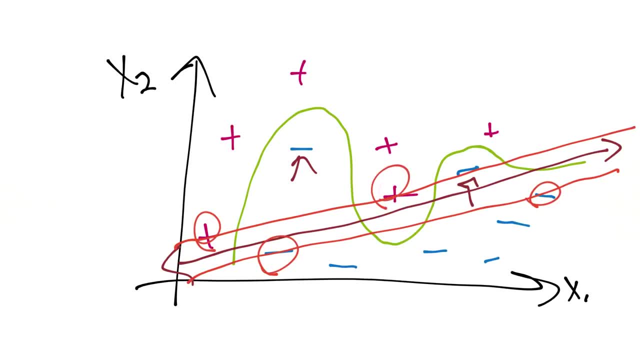 circled the support vectors. this time we have two here and two here, and this was dangerously close to being a support vector. but just understand, this is a toy problem. i've just kind of drawn it and not everything i've drawn is perfect, but anyways, uh. so in this case, right, you've got two support vectors on each side, four total support vectors. 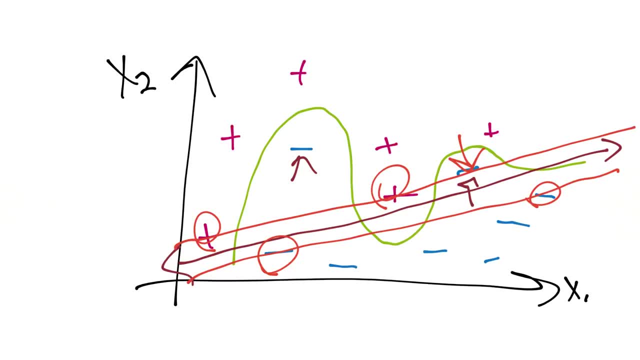 and we also have just plenty of data, data points here that are not support vectors, right? so much fewer of our data is or are support vectors, and that's that is, in theory, better, because you have less over fitment going on. so why is over fit? you know? 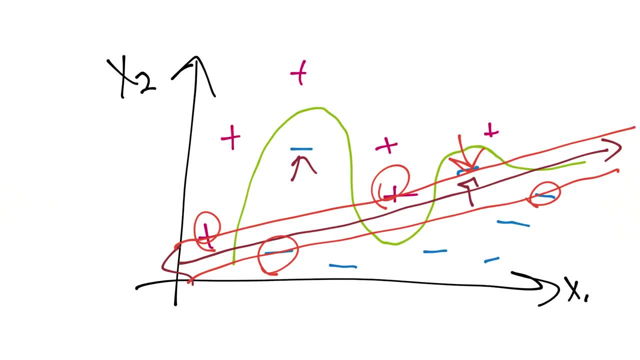 an over fitment is just a statistical thing, like that's just inherently bad. but what is going to end up happening? like if you over fit to historical data, it's just likely that in the future data you're just not going to be just right, because the future is going to have noise, it's going to 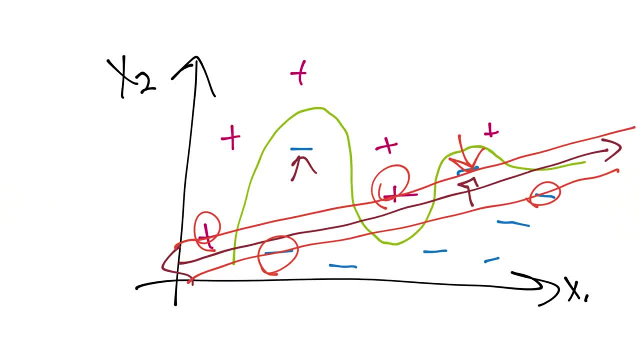 be different than the past data. so if you fit that past data perfectly, you're going to screw up in the future data. so you'll know this. though, if you do training and testing, which is something we've already covered up to this point, but the real question becomes: let's say, you train and then you test and you 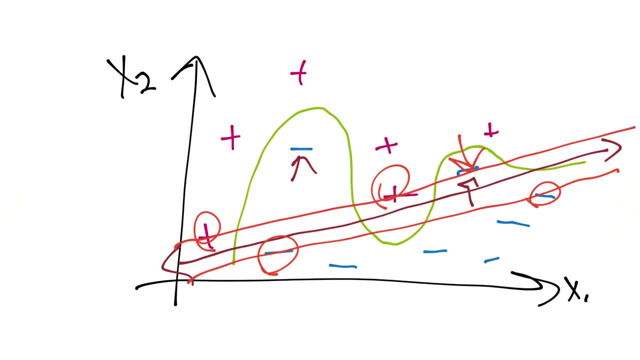 have 52 percent accuracy and you're like, wow, geez, that's, that's no good. and then you're kind of wondering, hmm, is are my, is my theory wrong? is this just something that's not going to work? or maybe should i use a different kernel or something like that, and you might not really. 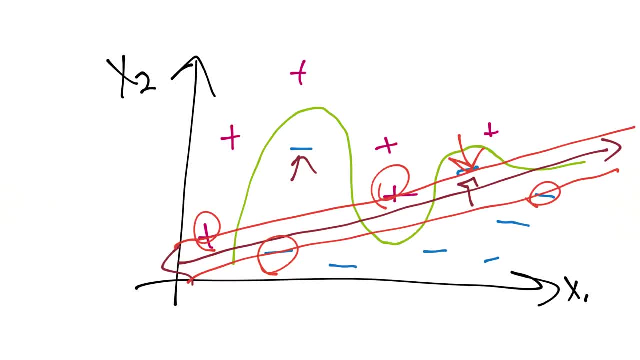 know, one thing you could do is take a shotgun approach and just use a different kernel, see what happens, right. but the other thing is that if you do training and testing and you're like oh my god, what's going on, and the other thing you can do is just query to see how many support. 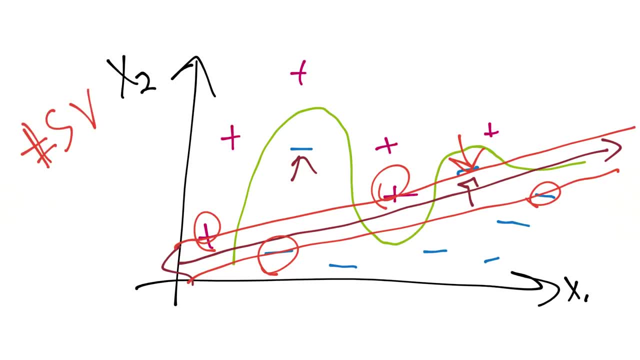 vectors do you have? so maybe number of support vectors, and then divide that by number of samples and if that's a large number, right, uh, you know, the closer to one that is, the worse off you are, and probably if you're in reality on a real data set, if you're more than you know, 10, let's say. 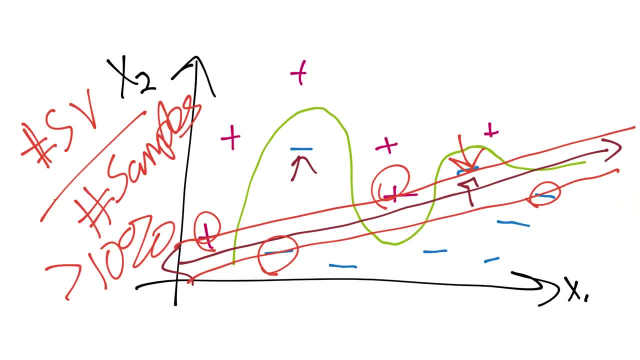 you've got more than 10 percent, you're going to have a lot of data set and you're going to have more than 100 data data points, uh, or feature sets, rather samples, whatever you want to call it. if you've got more than 100, probably 10 maybe. maybe you can go up to 20, but really probably 10 anything. 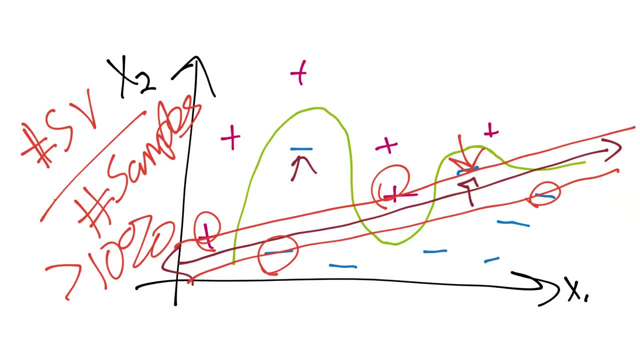 more than that. you. that should signal to you you've done some sort of overfitment. so it might not be the case that your data is not linearly separable. it might be the case, but you don't know yet. but maybe you should try, um, try a different, a different kernel, like, let's say, you, you come. 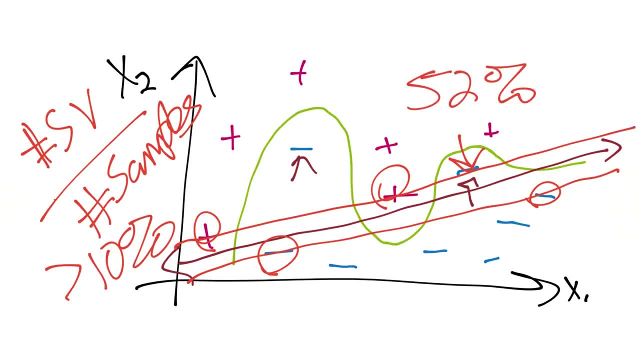 back with 52 percent accuracy. uh, 52 accuracy and uh, you have i don't know um 80 percent are support vectors. okay, if that's the case, you've got some overfitment going on. maybe try a different kernel. but if you've got 52 accuracy and only eight percent of your data is are support vectors, your data is probably not. 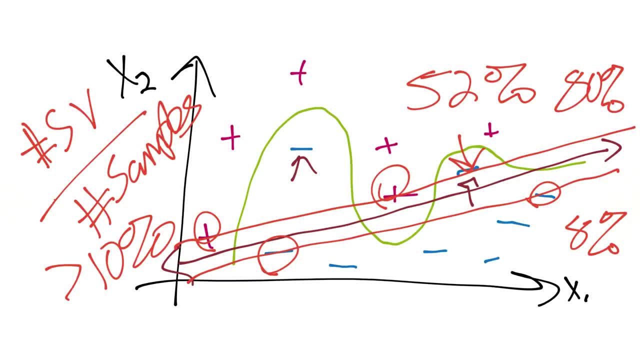 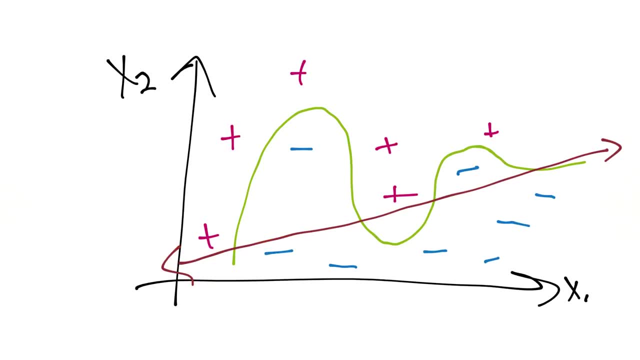 going to work out. you can still try a different. you know, you go ahead and try a different kernel, but but probably, uh, something else is right. so what we've got here, minus all of this mess, nice and clean. now, what we've got here is, when you have some sort of, let's say, a separating 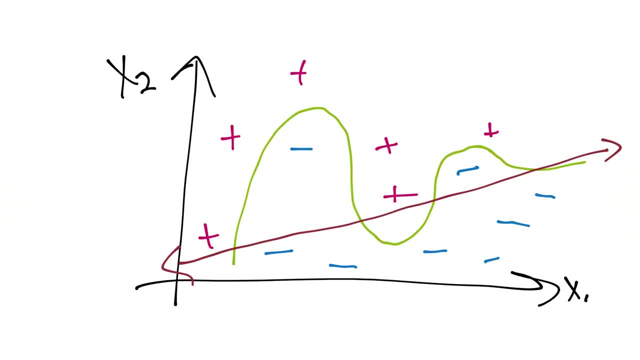 hyperplane where you actually have some data that is kind of in violation of that separating hyperplane. what you have is most likely a soft margin classifier. now, in this case, most likely we wouldn't accept a a soft margin all the way up to this point, so we're going to have to try a. 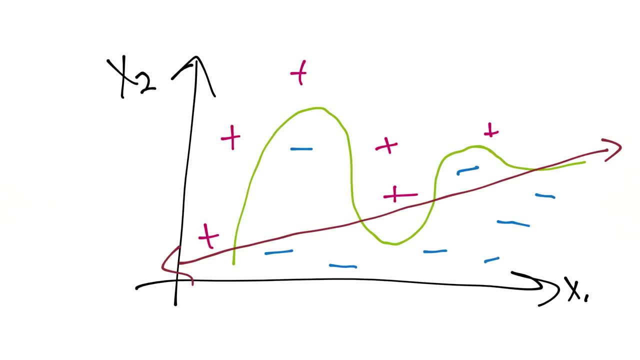 soft margin classifier at this point, uh, but keep in mind, this is just for a simple example, for now. so, um so, what's going to happen with a soft margin, a soft margin support vector machine, what you're going to have, as opposed to just by? obviously, it should be an intuitive here, but the other one, 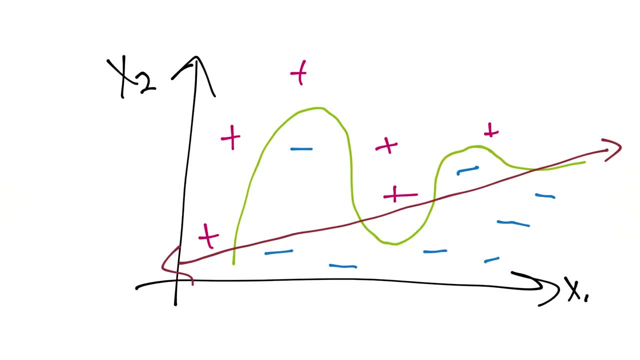 would just be a hard margin, like this green line. this is a, this is a hard margin classifier. right, that would be a hard margin and just like the rbf is kind of like the default kernel, it's actually the case that a soft margin classifier is going to be your default because, again, in the real world, a lot of your data is not going to be 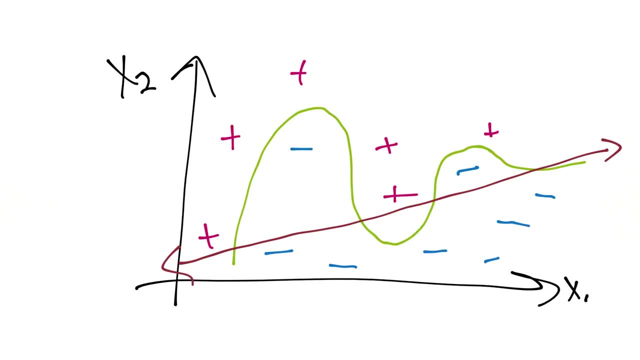 perfectly linearly separable, without some degree of overfitment. so, anyways, uh, so with, with, uh, with the soft margin, what you're going to have is you're going to have some sort of degree of error, right. so, so kind of like, with, with regression. you know the distance, right, uh, from the the 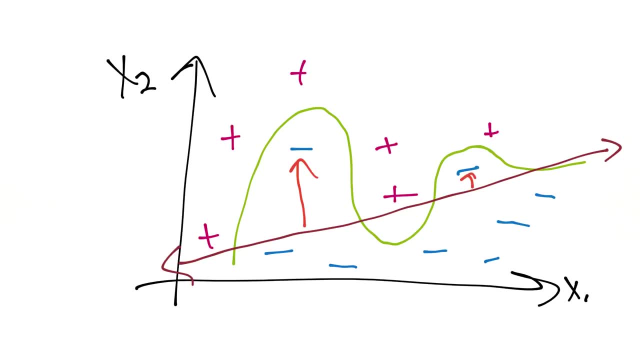 hyperplane. let's say to the data point: that's going to be your error, right, and and how might we? we allow some degree of error. well, we have what we call slack. okay, and what slack is going to be for us is, generally, we're going to denote slack, this little symbol, here, and what we're going to do is: 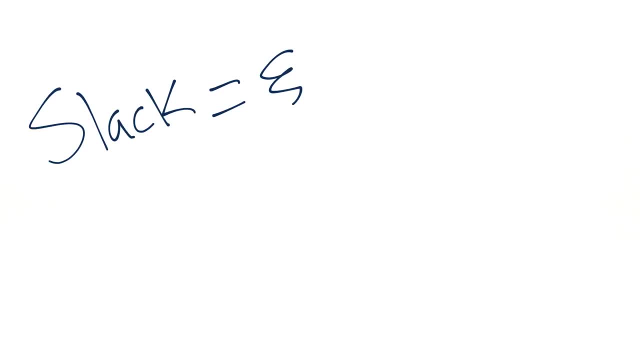 we're going to say: okay, remember before that constraint, basically where we were. we were saying that, uh, y sub i, x sub i, dotted with w plus b, and then it was: either minus one is greater than or equal to zero, but in this case let's say greater than or equal to one, okay, and in this case, uh, this was the. 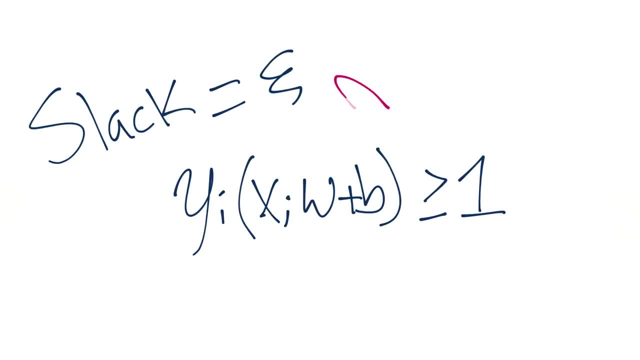 original kind of equation. but now what we can do is introduce this slack variable and say, okay, y sub i multiplied by x sub i dotted with w plus b really just needs to be greater than or equal to one minus our new slack variable, right? so so we're giving it some sort of leeway here now, of course, 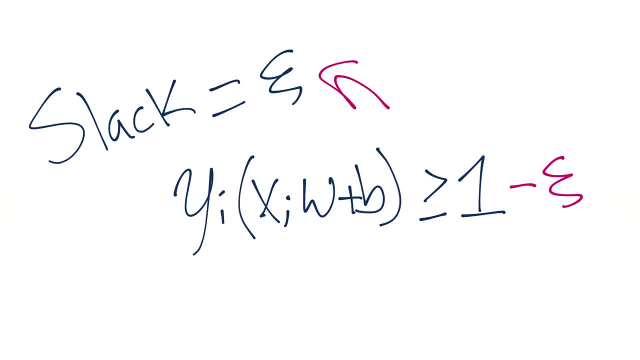 uh, it slack obviously needs to be. uh, let me just write it. uh, we'll just write it up here. right, slack must be greater than or equal to. i was almost going to write it in python terms, but anyways, it has to be greater than or equal to zero. right, it has to be a positive number, and if it was? 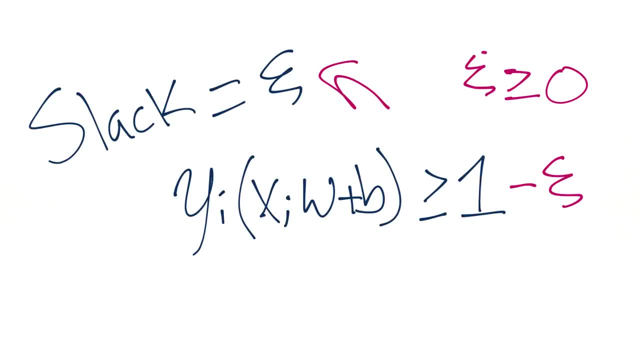 equal to zero, then that would just be hard margin. but the more slack you give it, the more soft your margin is going to wind up being. so now you might have, uh, total slack. so if we were going to say, hey, what is the the total slack? well, that would just be the sum of i over that slack variable of i, right it's. 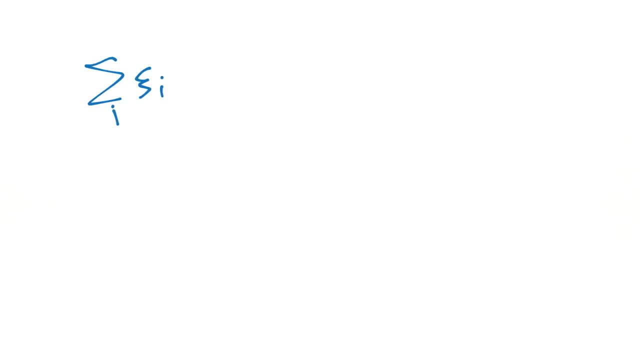 just the this: the sum of all the slacks. okay, so, yay, mathematic notation. so obviously we probably- you know you might want to, you might choose like, hey, yeah, we want to allow for some slack, but is it not kind of philosophically and logically correct that we probably want? 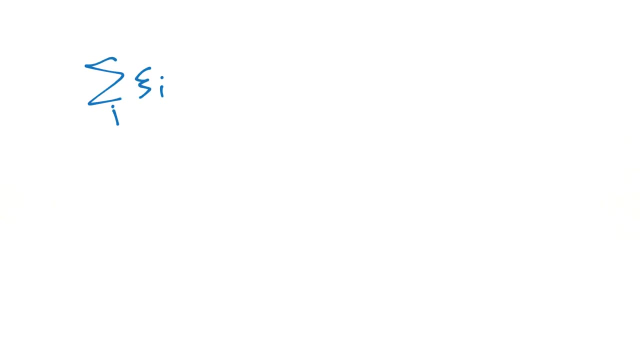 as little slack as possible. right, we, we would want to minimize the slack and obviously that's- you know, that's a scary, a scary turn to be thrown around here. but, yes, we, we really probably want to actually minimize the slack and we're going to want to minimize the slack and we're going to want to. 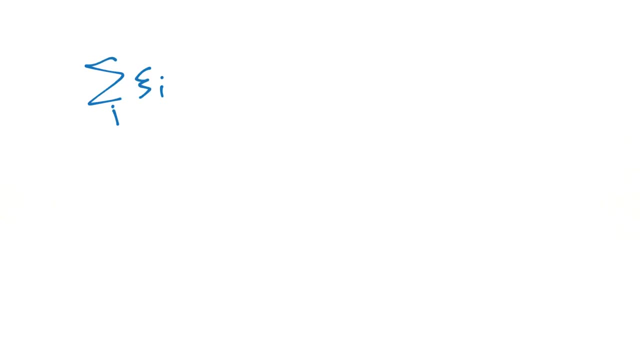 minimize the slack. so so how? how do we throw that into our actual equation? remember, in the, in the old days when we actually did the formal calculation of the support vector machine, we wanted to minimize, not mimmy minimize, and we wanted to minimize what. we want to minimize the magnitude of vector. 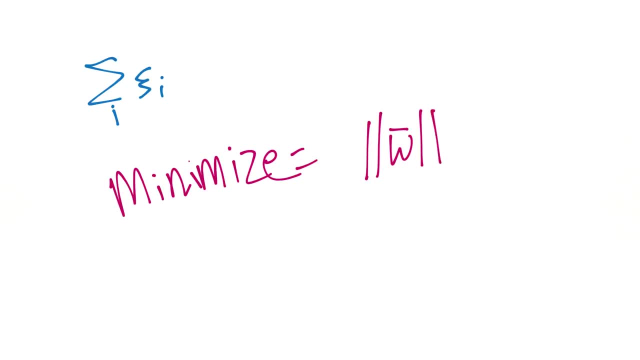 w. and then we said, just for ease of quadratic program, maybe we also, since you want to盾 minimize the magnitude of vector w, you also want to minimize the one half of the magnitude of vector w. squared right, that's just. you know, that just works. so then what you're going to do is you're. 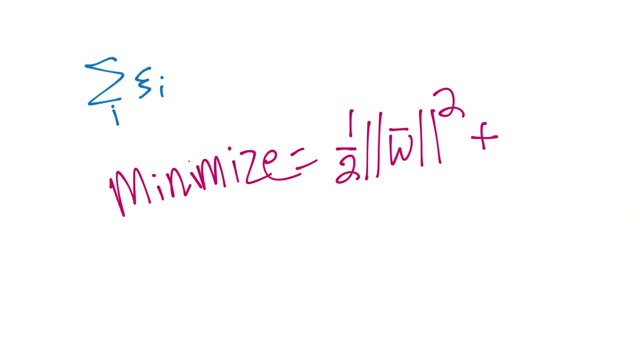 going to say plus, and then you're going to do this, this new thing that we just have right here: the sum of i over the total slack, basically the total sum of of all the slacks. so now you're going to have the sum of slacks, i and i, and then you're going to 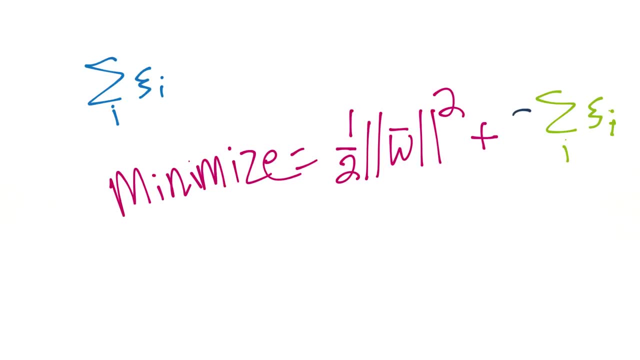 have this new value, and this new value is c. so now, before it was just to minimize this, but now it's actually we want to minimize all. we want to minimize all of this. okay, so we've already explained what slack is, we already know what the i's are, we already know the sum of all the slacks. 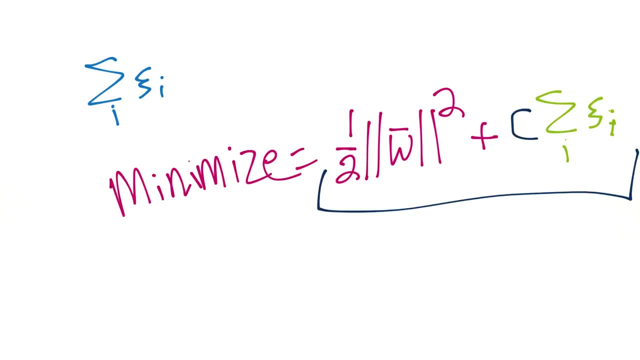 and stuff. so what is c? i mean just kind of looking at this equation, we want to minimize one half. basically we know we want to minimize the magnitude of vector w. okay, we already kind of know what that's going to do. and then we want to, but really we want to minimize. now we're trying to minimize this whole equation, so no longer are. 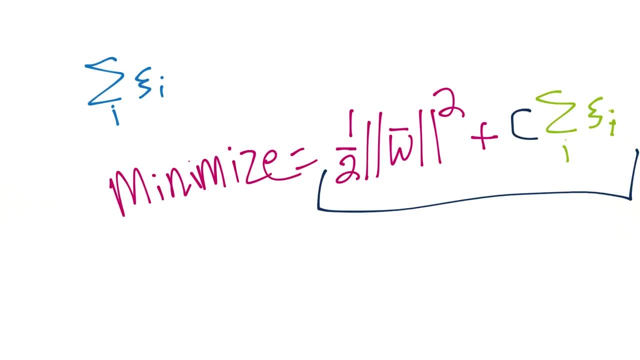 we just trying to minimize the magnitude of vector w. we're trying to minimize the magnitude of vector w plus c times all of our slacks right, add it up, okay. so sometimes, a lot of times, people are very confused of what c actually does. but if you look at this, this optimization problem, it should be. 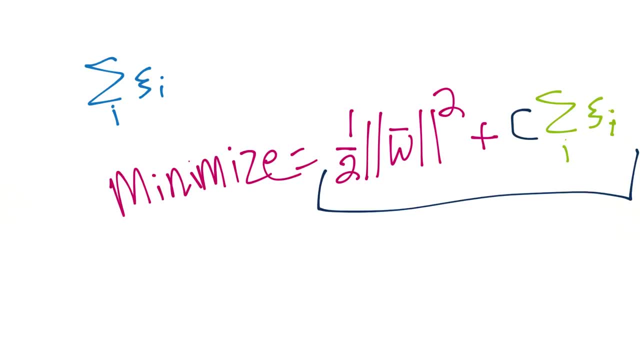 pretty obvious like: what if we? what if we raise? what if we raise the value of c? here? well, if we raise the value of c, we're saying we want less violations, because there's really no way, like if we're going to try to minimize this equation, the more we raise c, the more we're going. 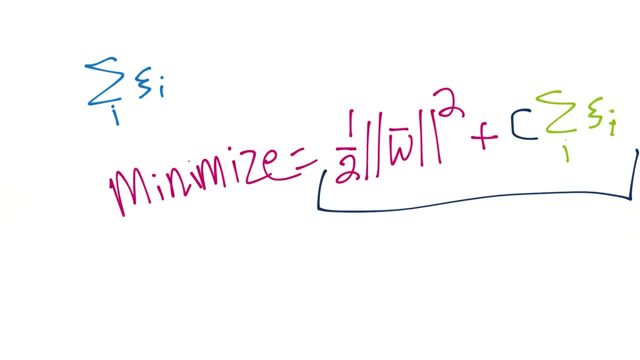 to punish for violations of the margin, and if we lower c, we're going to be more allowing of violation, because you can just, you can just see, like right, if you, if you raise the value of c, that's multiplying this right here. so that's just making the equation much larger. and so another way. 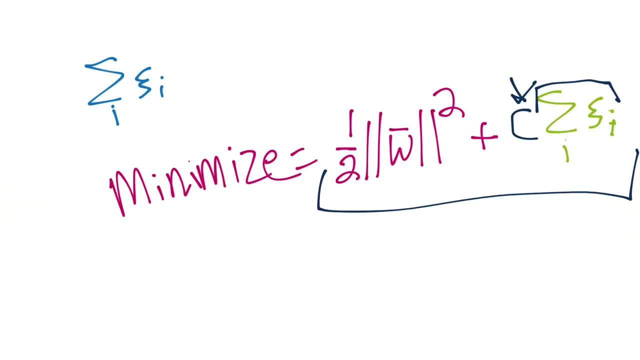 to kind of look at the value of c is to because, obviously, as you, as you, as you change c, like c and slack and all of those things, have absolutely no relation to the magnitude of vector w. so except in this, this little minimization, requirement, optimization problem, so so because of that, c is actually kind 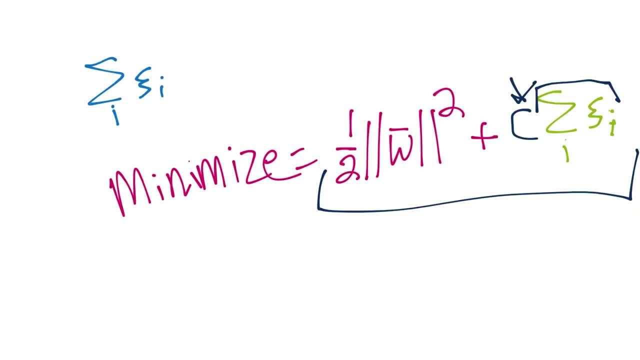 of like: um, it's where you get to decide how important slack is in relation to minimizing the magnitude of vector w right? so it's kind of your way of of kind of teeter-tottering between you know, whatever personal values you might have in the specific example that you're running. 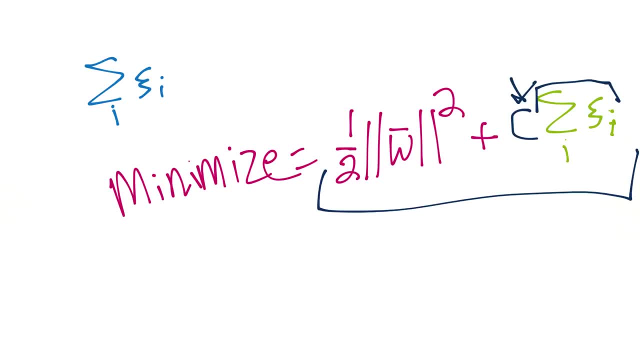 so c is something that you're going to be able to minimize, and you're going to be able to minimize it. you're going to kind of set as a hard. you're going to say, okay, i want c to be equal to one or five or 0.5 or 0.2 or whatever, and obviously the smaller you make c, the less it you know, the less. 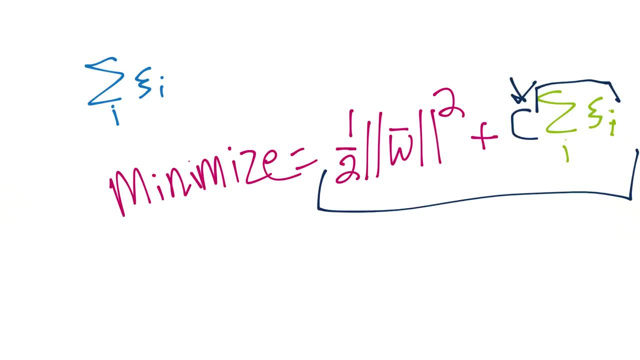 it matters what the slacks are right, the less it matters what those errors that violation, the less it matters. right, because the smaller you multiply this, these, you know the, the sum of all of the slacks, the smaller that is you're. you're minimizing the equation, right, just by changing c a little bit. 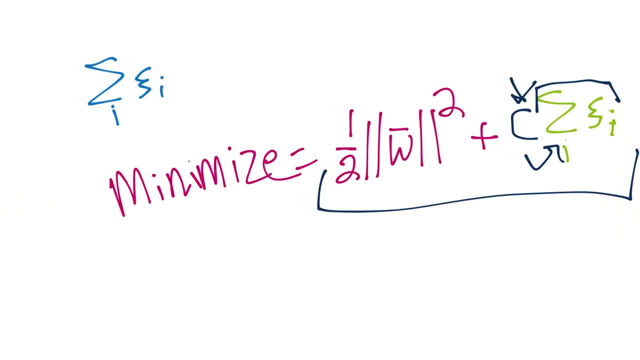 uh, so that is what c is, that's what slack is and that's kind of what. uh, that's what the soft margin classifier is doing. and, again, the kind of purpose of a soft margin classifier is so you don't overfit your data and in most cases, that's what you're actually going to be running is a soft. 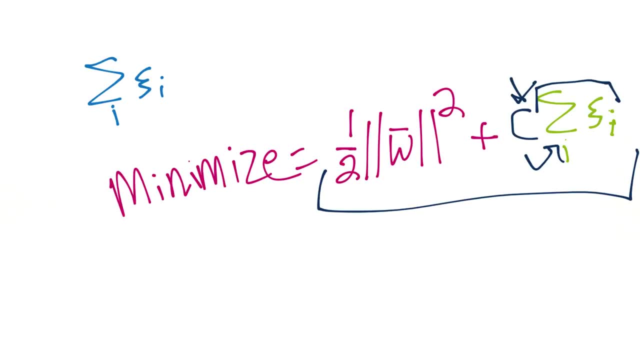 margin classifier because, uh, most real examples are just simply not linearly separable and if you take it to the number of dimensions required to make it linearly separable, you've probably done some over fitment. so you know one way you can kind of test this and compare it.